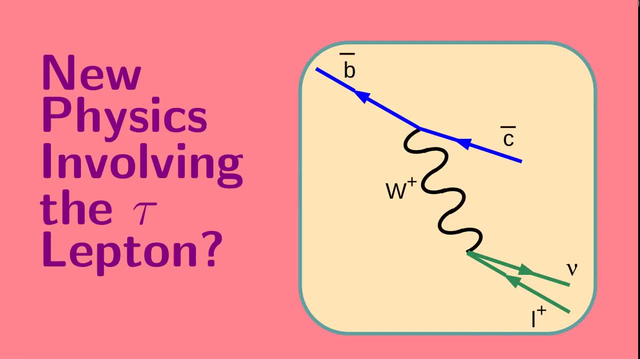 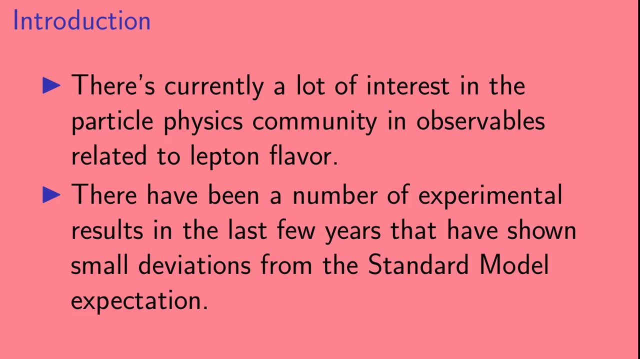 Hi, welcome to new physics involving the tau lepton. So there's currently a lot of interest in the particle physics community in observables related to lepton flavor. There have been a number of experimental results in the last few years that have shown small deviations from the standard. 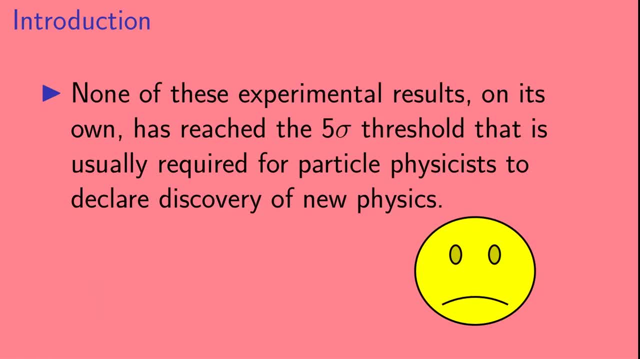 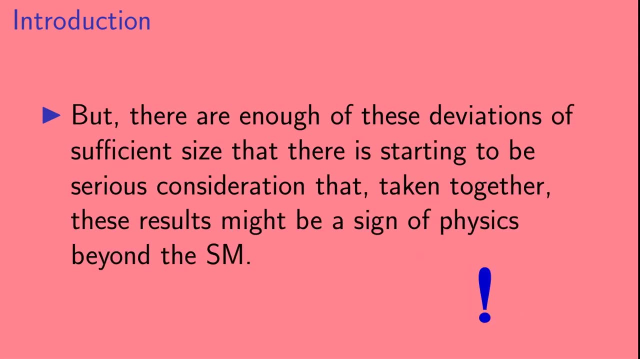 model expectation. Now, none of these experimental results on its own has reached the five sigma threshold that is usually required for particle physicists to declare discovery of new physics. But there are enough of these deviations of sufficient size that there is starting to be serious consideration that, taken together, these results might be a sign of physics beyond the 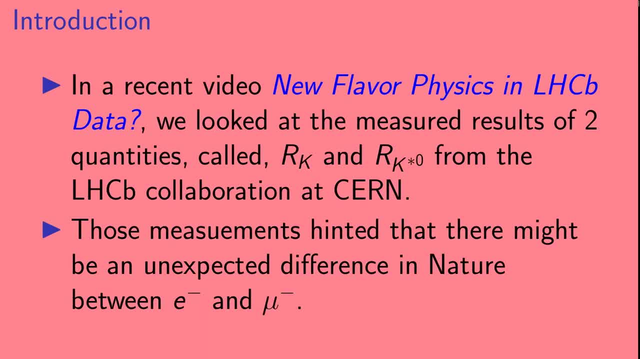 standard model. So in a recent video called new flavor physics in LHCb data, we looked at the measured results of two quantities called Rk and Rk star from the LHCb collaboration at CERN. Those measurements hinted that there might be an unexpected difference in nature between the electron and the muon. 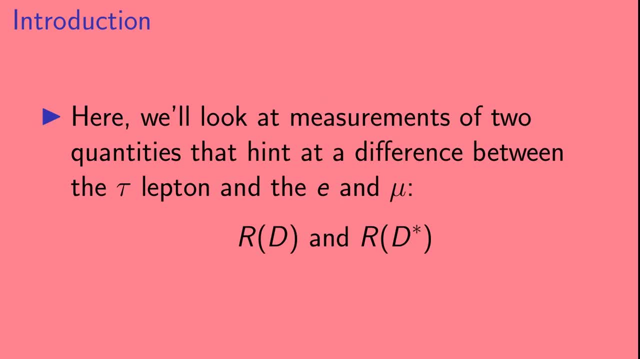 So in one of the recent videos we looked at the measured results of two quantities called Rk and Rk BOZ and a more comprehensive black electronic Тогда flígen, a very통licious схord just related- And plumbing in physics, along with basic manufacturers and climate law. 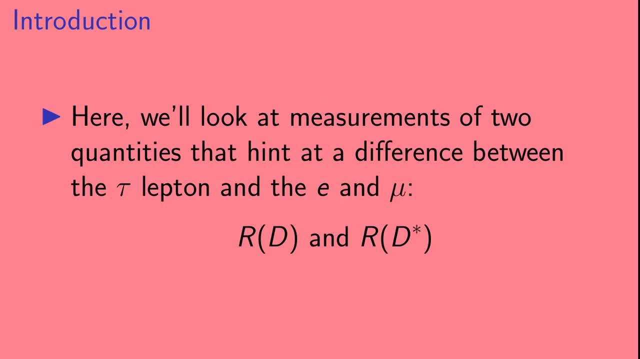 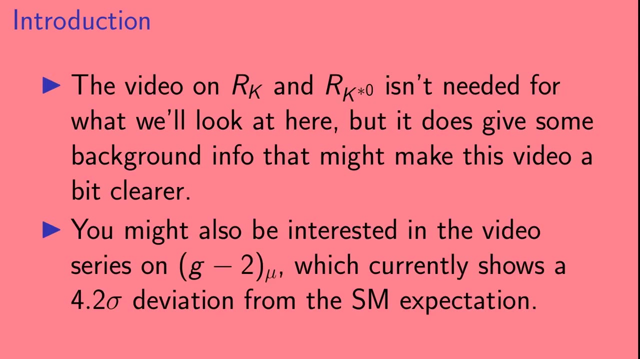 Here we're going to look at measurements of two quantities that hint at a difference between the tau lepton and the electron and mu, and those two quantities are called Rd and Rd star. Now, the video on Rk and Rk star isn't needed for what we'll look at here, but it does give some background info that 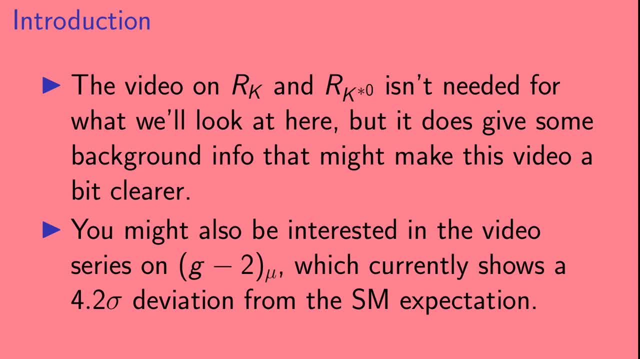 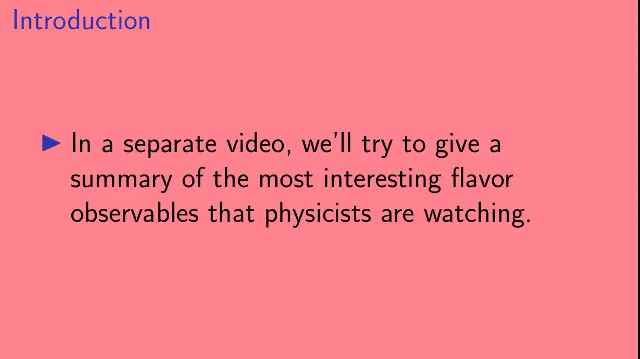 might make this video a bit clearer. You might also be interested in the video series on muon g-2, which currently shows a 4.2 sigma deviation from the standard model expectation. Also in a separate video we will try to give a. 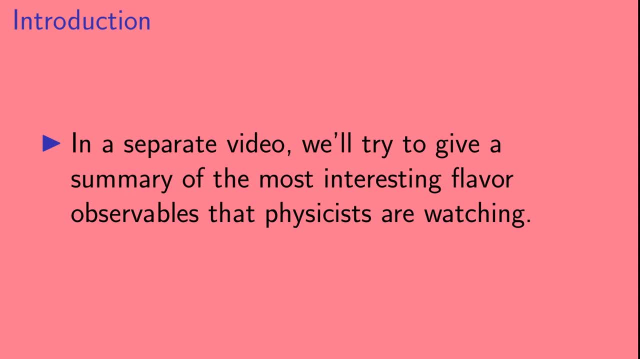 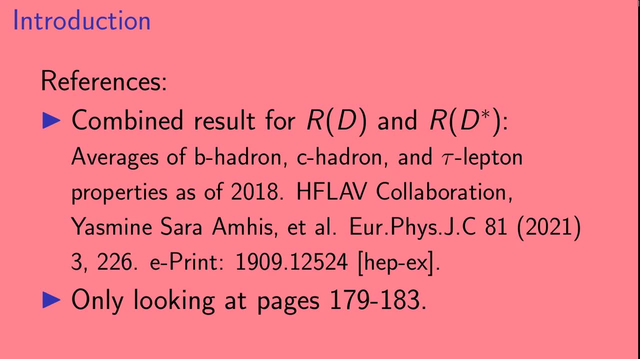 summary of the most interesting flavor observables that physicists are currently taking a look at. Okay, so let's mention a few references. So the combined result for Rd and Rd star that will be given at the end of the video is being taken from a paper from 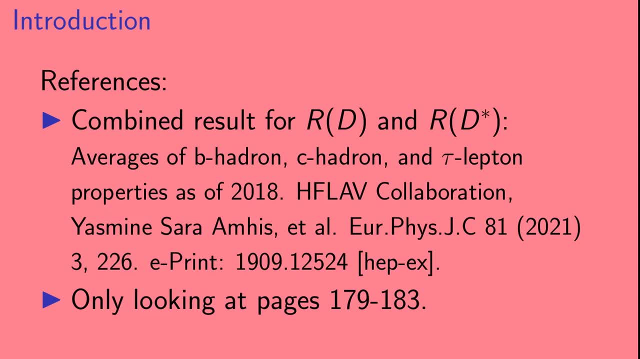 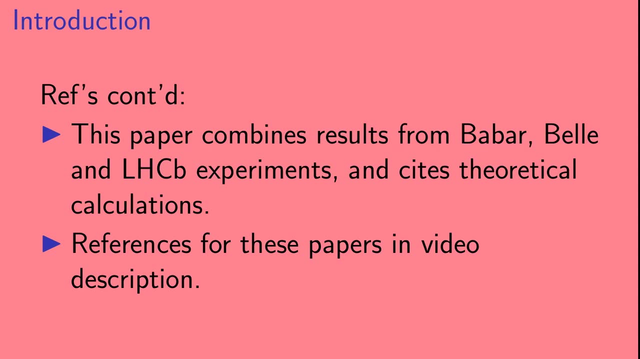 the heavy flavor averaging group, and this paper is a 494 page behemoth and we're only going to be looking at pages 179 through 183.. Now that paper from the heavy flavor averaging group combines results from the Babar-Hansel-Hansel. 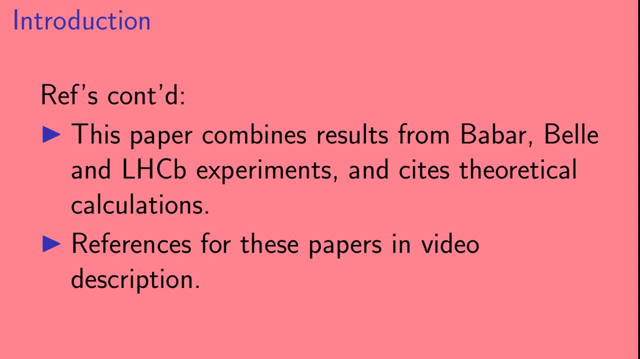 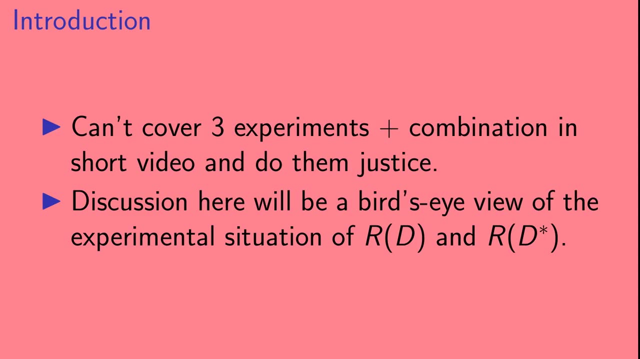 experiment with the Rd-Bell-LHCb experiment, and it also cites theoretical calculations. The references for those papers you can find in the video description below. Now we should say upfront that it's not possible to cover three experiments and the combination of the results in a short video and do them. 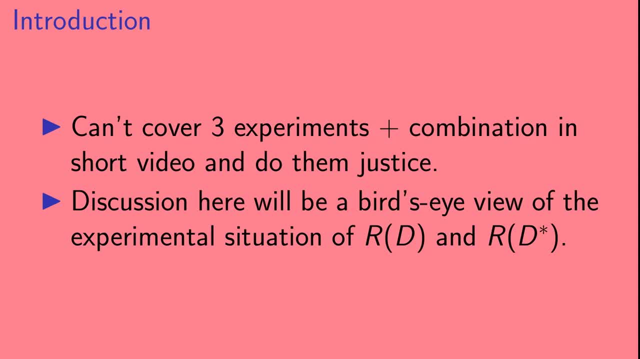 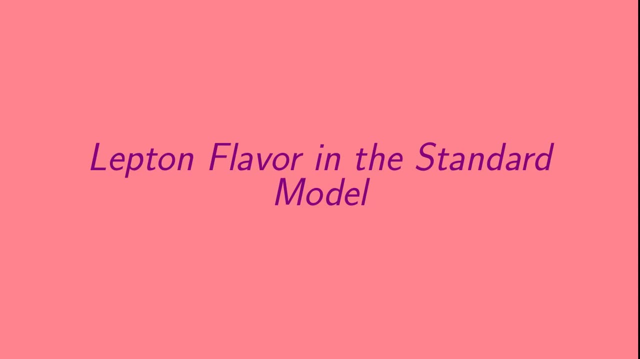 justice in any significant way. So the discussion here is definitely going to be a bird's-eye view of the experiments. Okay, so we're done with the experiment. so let's move on to the next experiment. We'll start our experimental situation of Rd and Rd star. Okay, so with that, let's. 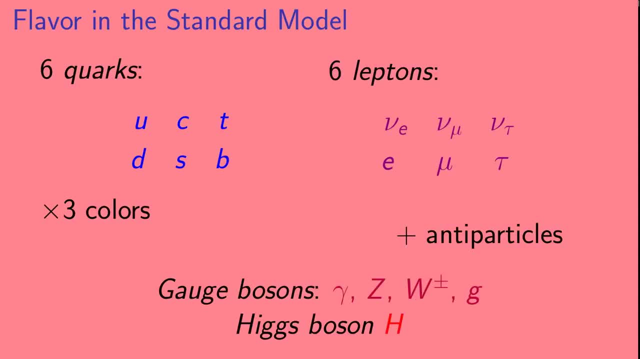 very briefly talk about lepton flavor in the Standard Model. Okay, so in the Standard Model of particle physics we have six quarks and six leptons, and these quarks and leptons interact with the gauge bosons of the Standard Model. so 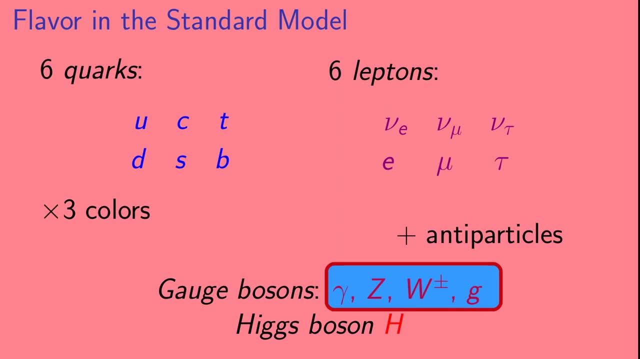 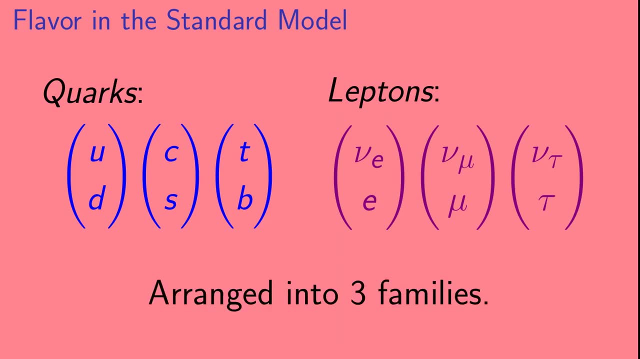 and the gluons, And also there's the Higgs boson. Now the quarks and leptons are arranged into three families, and these families are identical except for mass terms of the quarks and leptons. Now, in the standard model, the three 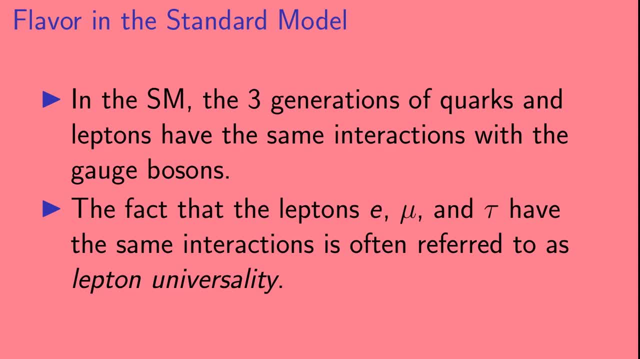 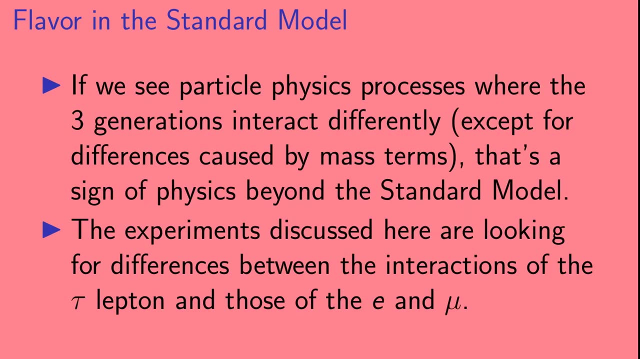 generations of quarks and leptons have the same interactions with the gauge bosons, And the fact that the leptons, the electron, the muon and the tau have the same interactions is often referred to as lepton universality. So if we see, 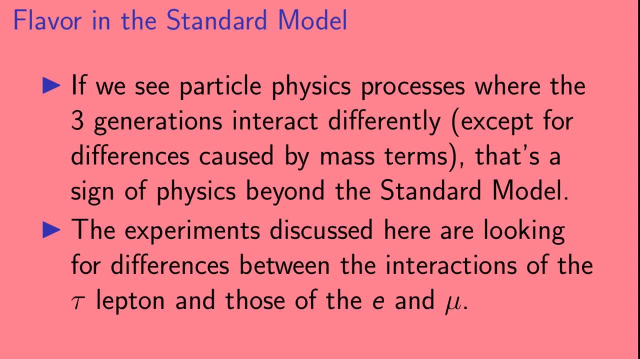 particle physics processes where the three generations interact differently, except for differences caused by mass terms. that's a sign of physics beyond the standard model, And the experiments discussed here are looking for differences between the three generations, between the interactions of the tau lepton and those of the electron and 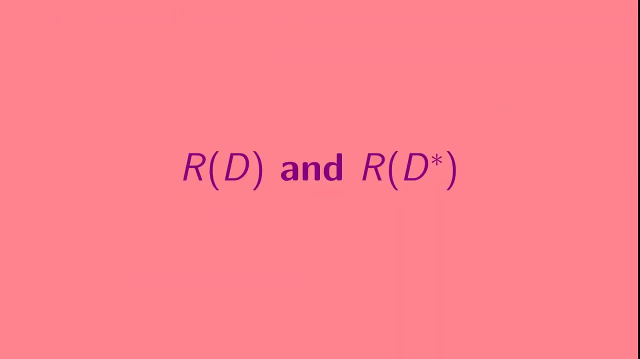 muon. Okay, so with that we can start to talk about Rd and Rd star, And in fact we're mostly just going to talk about Rd, because Rd star works almost exactly the same way. So let's take a look at a particle called a B meson. It's not a fundamental 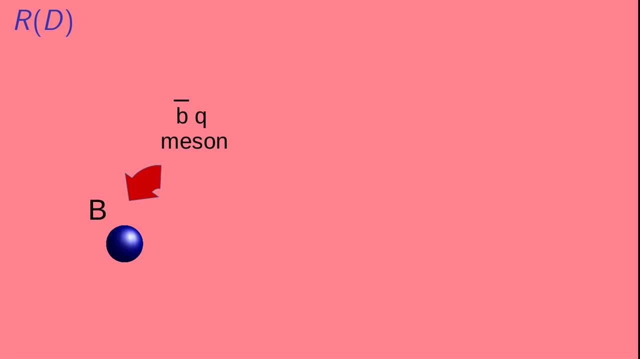 particle. It is made of a quark and an anti-quark. The anti-quark is a B anti-quark, which we denote B bar. We'll talk about the identity of the quark in just a moment. Now, in the standard model, a B anti-quark can turn into a C. 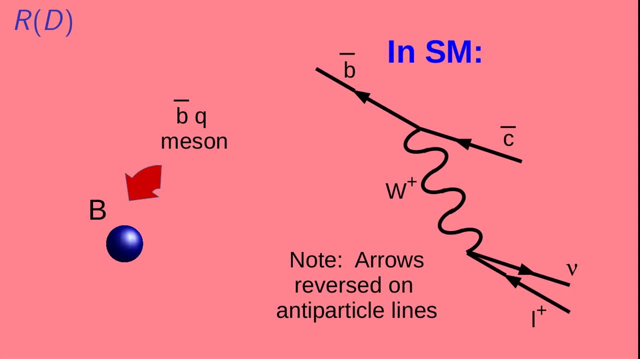 anti-quark by emitting a W particle which then can decay into a positively charged lepton, which we'll call L, and a neutrally charged lepton, which is a, C And a neutrino. So this gives the process: B bar goes to C bar plus a positively. 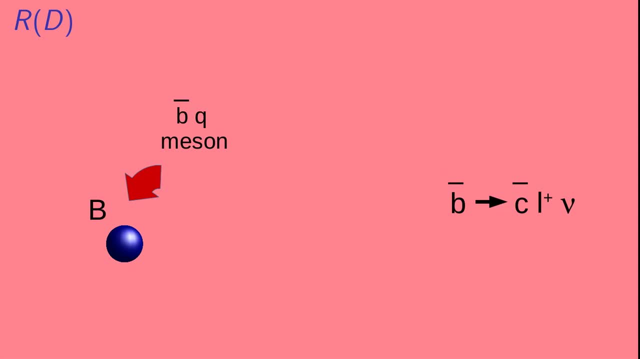 charged lepton and a neutrino. Let's apply this process to our B meson. The B anti-quark in the B meson turns into a C anti-quark and a positively charged lepton and a neutrino are equal. The other quark just goes along for the ride, forming what we will generically. 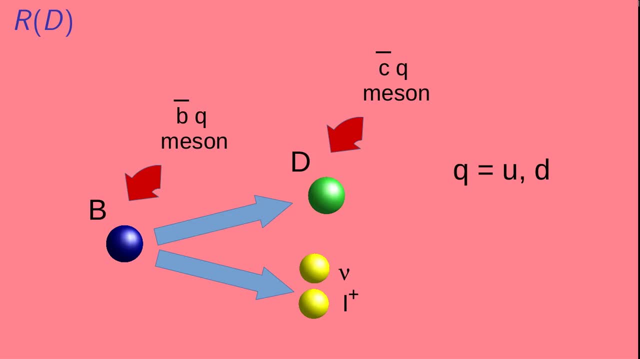 call a D meson. Now, when people talk about B mesons, they typically are referring to the case where the other quark is an up quark or a down quark. If it's an up quark, the B meson is a positively charged B plus and the D is a. 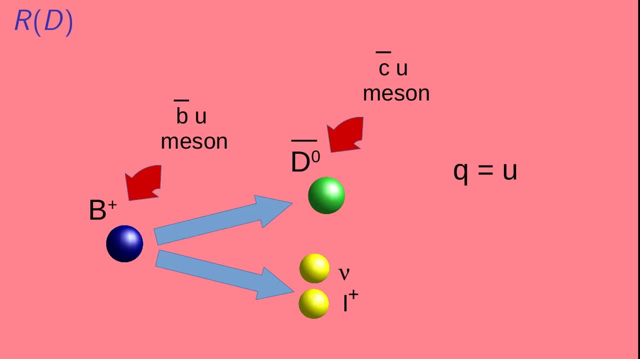 neutral particle called a D zero bar. If the quark is instead a down quark, the B meson is a B zero and the D meson is a D minus. Also, we're going to include processes where every particle in this diagram is replaced with its anti-particle. So the cartoon we've 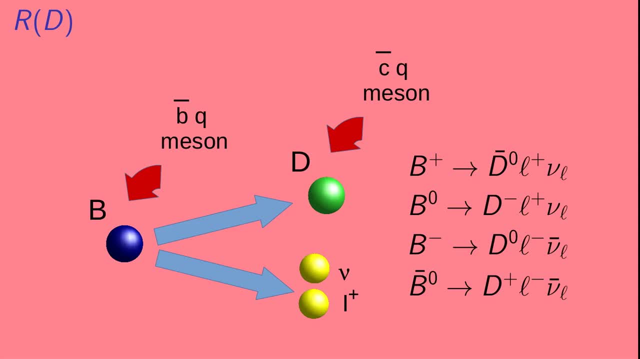 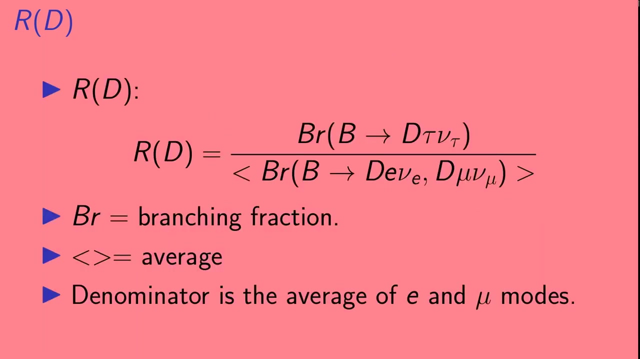 drawn here actually represents four different decays, depending on what type of B meson you're starting with. We're going to refer to all of these processes generically as B goes to DL nu. Okay, so now we're ready to talk about the definition of Rd. RD is the ratio of 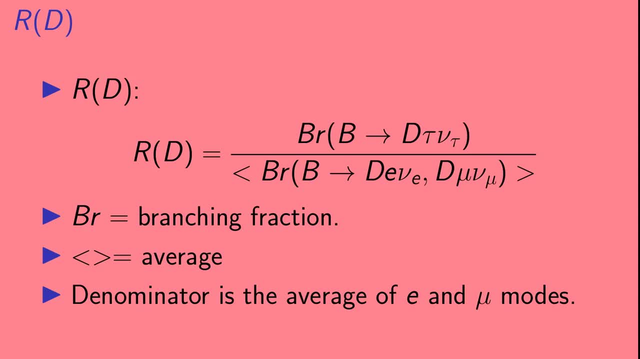 the branching fraction of a B meson to a D meson and a Tao lepton and a neutrino to the branching fraction of a B meson to a D meson meson and either an electron and a neutrino or a muon and a neutrino. The 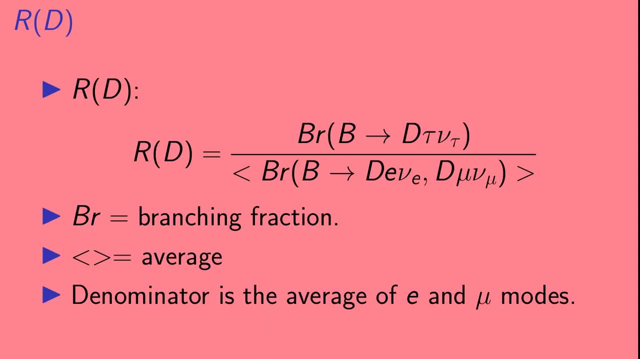 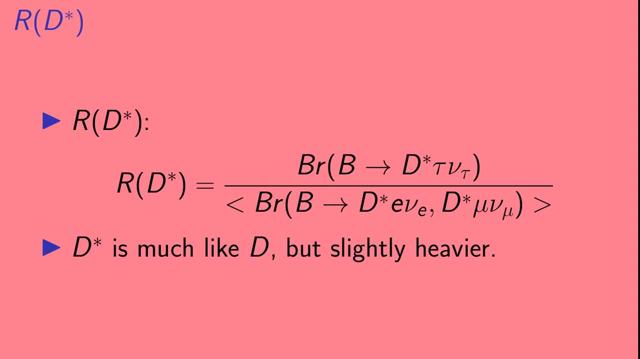 branching fraction is just the fraction of the time that a B meson decays in that particular way. The denominator is the average of the electron and muon branching fractions. Rd star is the same, but the D meson is replaced with a different meson called D star. it is very similar to a D meson, but 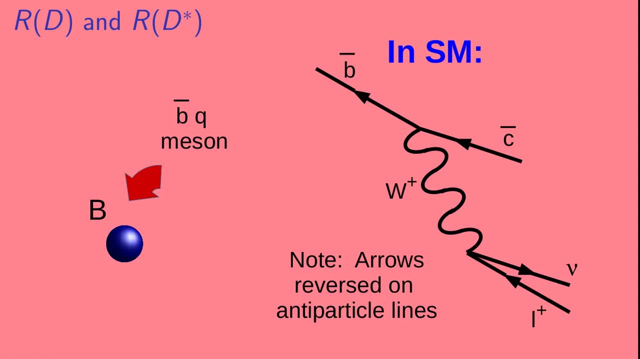 slightly heavier. OK, so now let's look back at that diagram which mediates these decays that we're interested in in the standard model. In the standard model, the W boson has the same interaction between the three types of leptons: the electron, the muon and 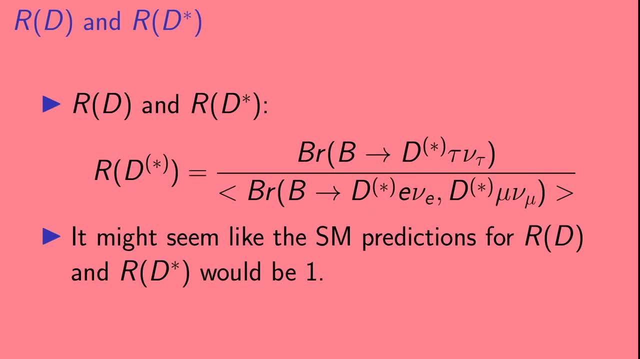 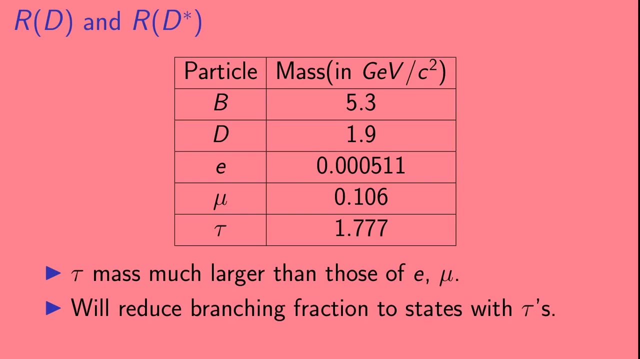 the tau, So it might seem like the standard model prediction for Rd and Rd star would be 1.. However, the tau is much heavier than the electron or muon. This will actually reduce the branching fraction to states with taus and make Rd and Rd star much less than 1.. 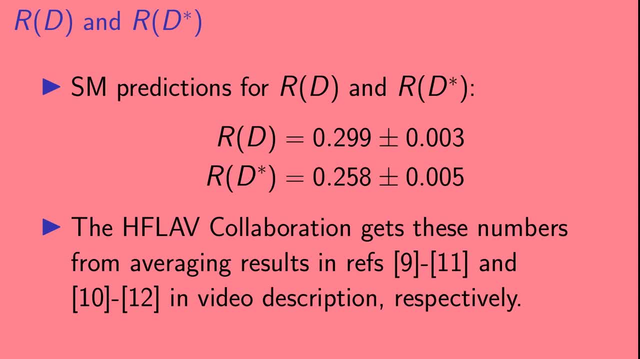 The standard model predictions for Rd and Rd star used by the heavy flavor averaging group are 0.299 ± 0.003 and 0.258 ± 0.005, respectively. They get these numbers from averaging results in references 9-11 and 10-12. 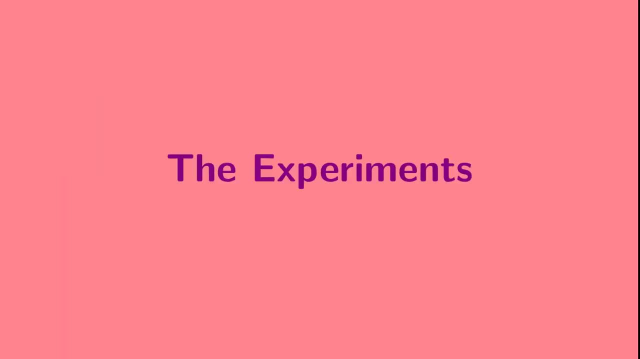 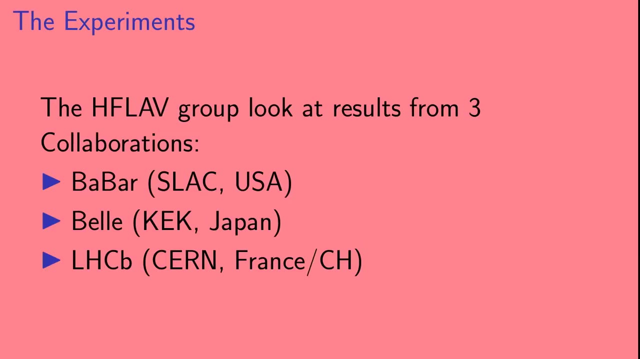 that you can find in the video description. Okay, so now we're ready to talk about the experiments: The heavy flavoring, The heavy flavor averaging group. look at results from three collaborations: Babar, which was based at SLAC in the USA. 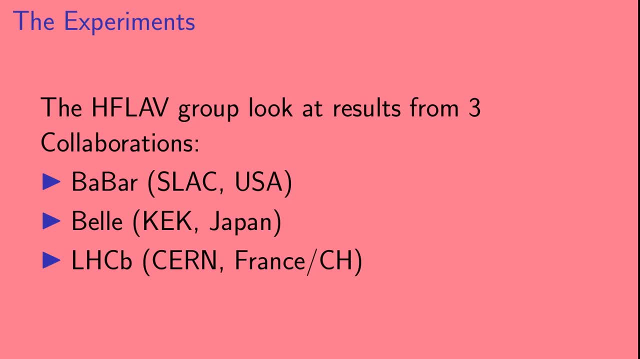 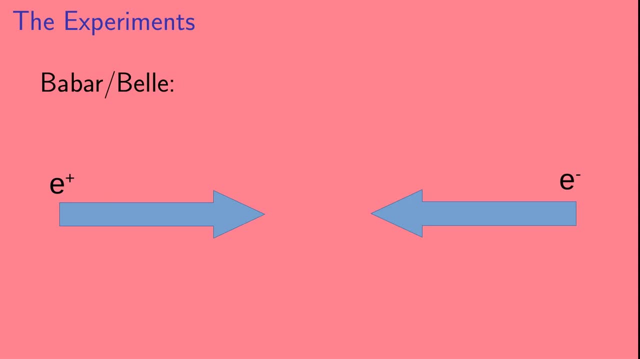 Bell, which was at Keck in Japan, and LHCb, which is at CERN on the French-Swiss border. Now Babar and Bell collide electrons and positrons. They collide them at a center of mass energy of 10.58 GeV. 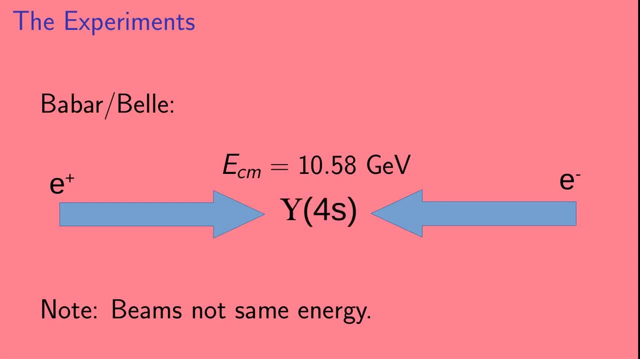 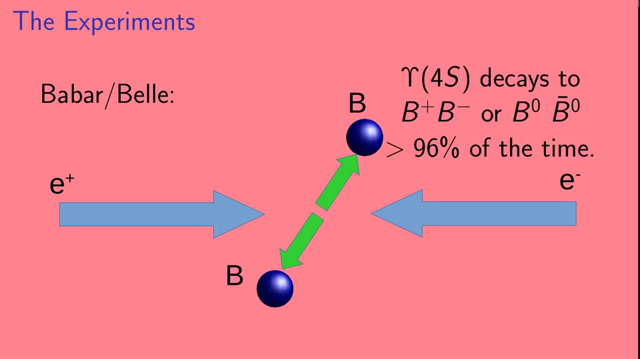 At this energy you can produce a particle called the Upsilon-4S. Babar produced 471 million of these Upsilon-4S particles, and Bell produces 772 million of them. Now the Upsilon-4S particle decays to either charge or neutral B-Maison. 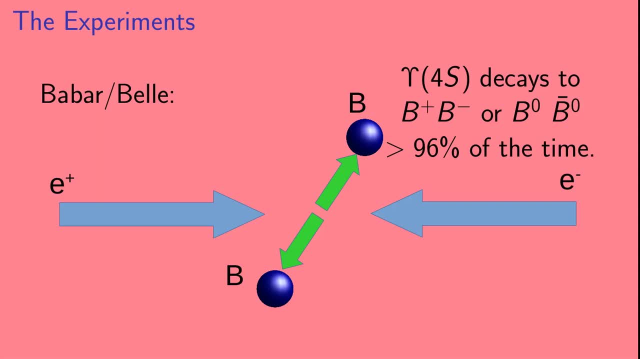 Now the Upsilon-4s particle decays to either charge or neutral B-Maison more than 96% of the time. So Babar and Bell produced a lot of B mesons. Then they look for one of these B mesons to decay to D or D star L nu. 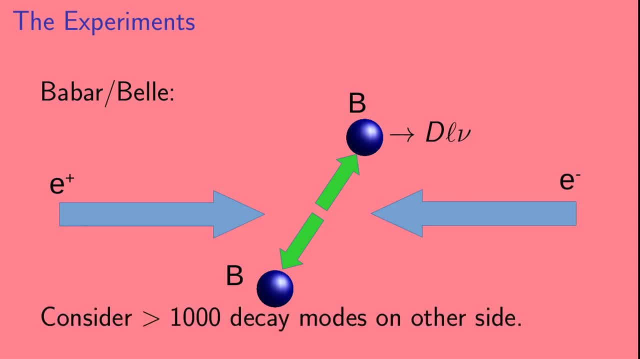 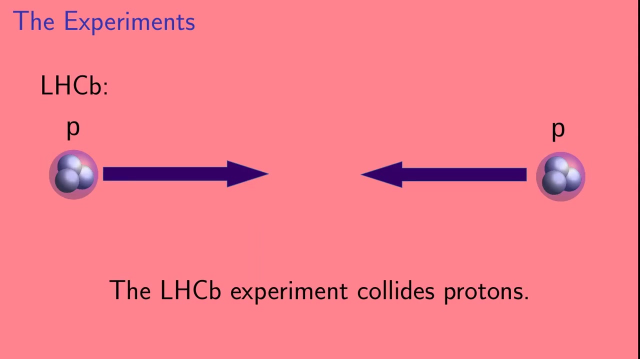 However, that's not the only thing that a B meson can decay to, so they actually consider over a thousand different decay modes that can happen to the B meson on the other side of the event. Okay, so now LHCb. So LHCb collides protons and in. 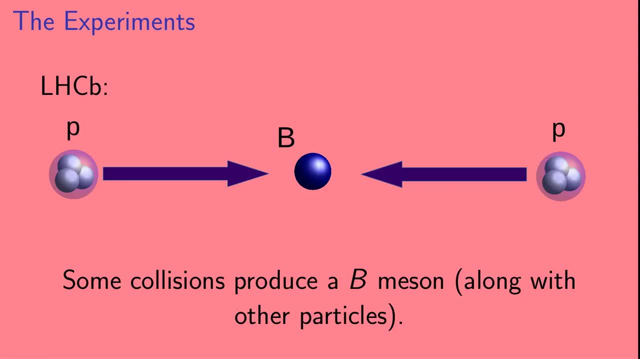 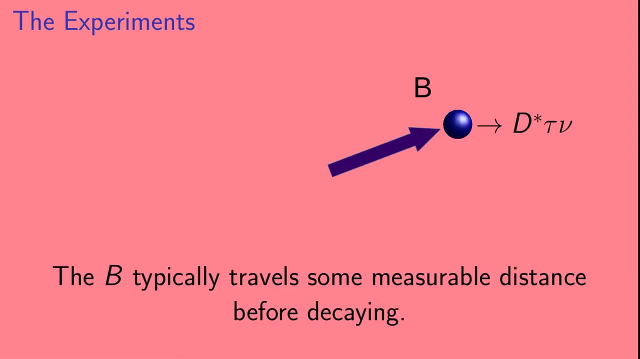 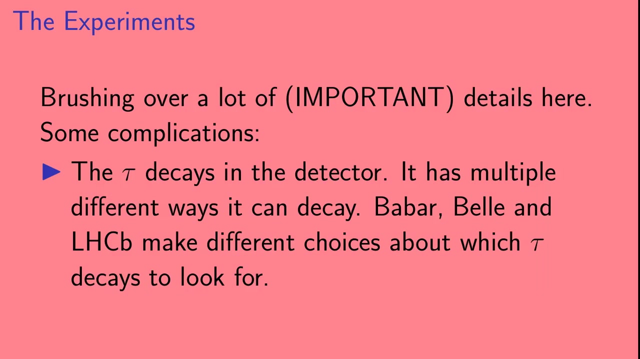 some of these collisions you'll produce a B meson along with some other particles. The B meson typically travels some measurable distance before decaying and then LHCb looks for the decay of that B meson going to D star tau nu. Now, here I'm brushing over a lot of very important details, so I'm going to briefly. 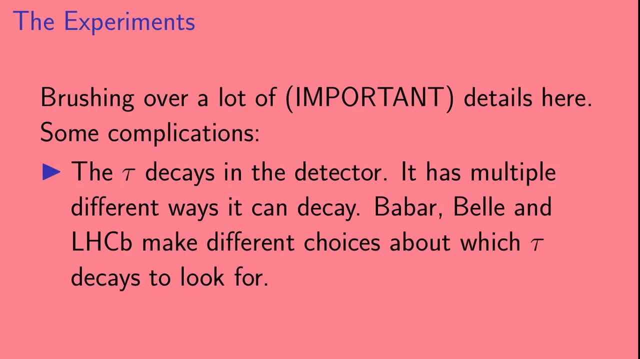 mention some complications here. So the tau lepton actually decays in the detector. It has multiple different ways that it can decay and Babar Bell and LHCb make different choices about which tau decays to look for in their detector. 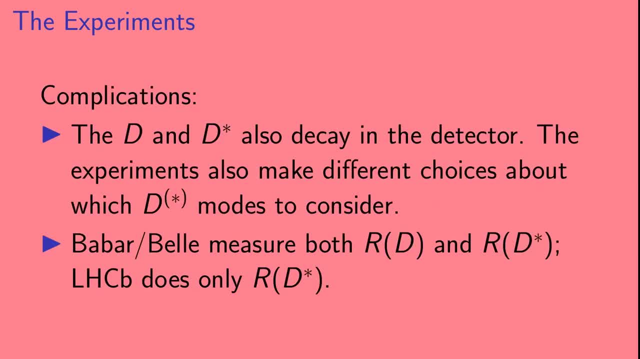 Also the D and D star also decay in the detector. The experiments also make different choices about which D and D star modes to consider in their experiments, And Babar and Bell both measure Rd and Rd star, whereas LHCb only looks at Rd. 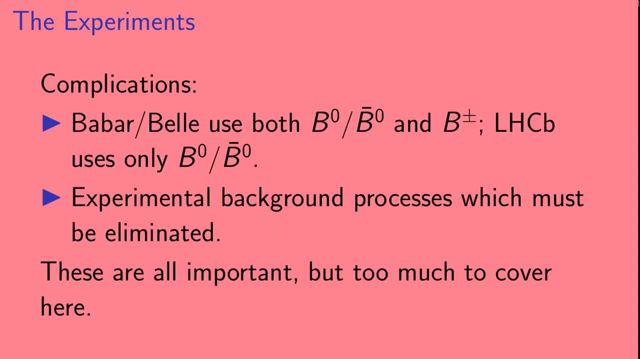 Okay, And finally, one very important fact is that there are also experimental background processes which have to be eliminated from your data. So these are processes that are not the process that you're looking for, but that can look like it and be mistaken for it. 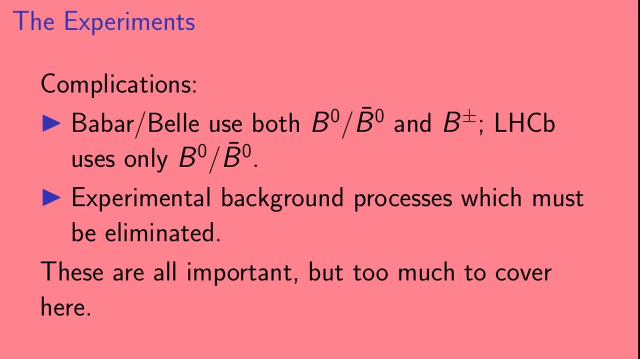 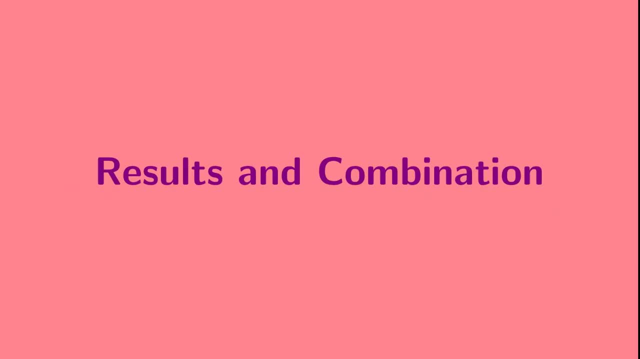 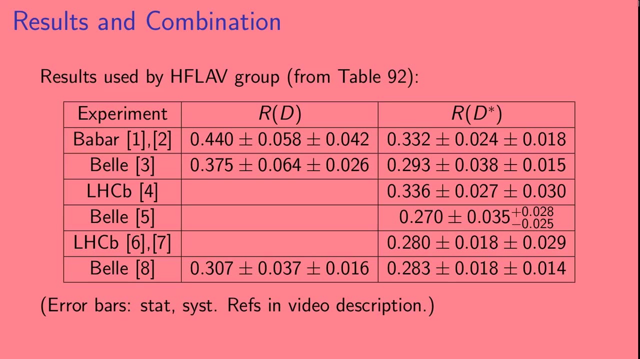 All of these issues are important, but they're far too much to cover in this short video. Okay, so now we can take a look at the results and combination. Okay, so here are the results from Babar Bell and LHCb that are used by the heavy 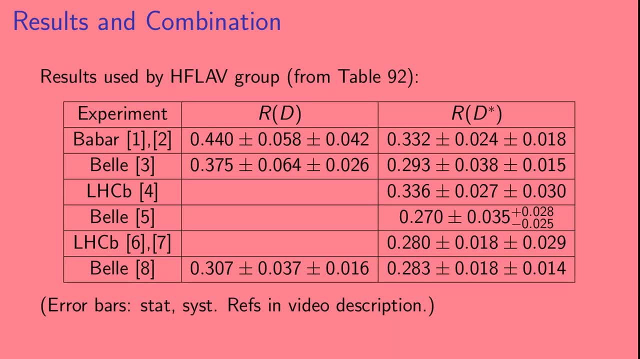 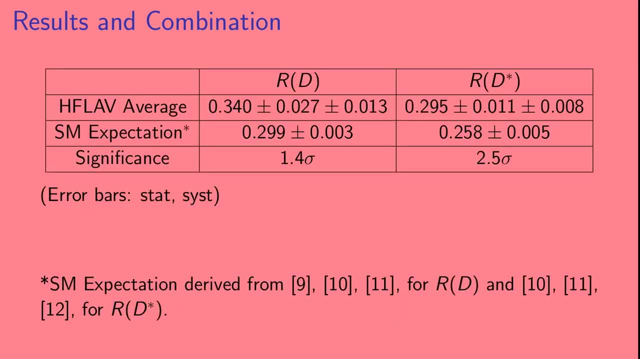 flavor averaging group. These numbers are just taken from table 92 in the heavy flavor averaging groups paper. Now the heavy flavor averaging group gets an average of those values for both Rd and Rd star and those values are shown here. They then compare them to the standard model expectation and get a significance. 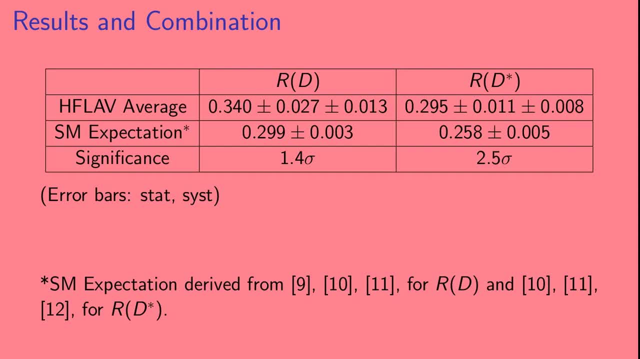 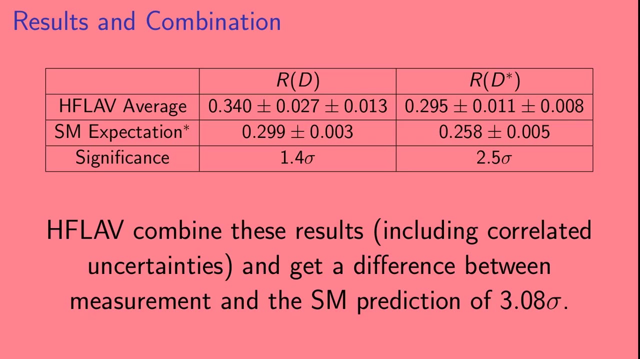 They find that Rd is 1.4 sigma above the standard model expectation and Rd star is 2.5 sigma above the standard model expectation. Now the heavy flavor averaging group combine these results, including correlated uncertainties between the different experiments and between Rd and Rd star, and they get a difference. 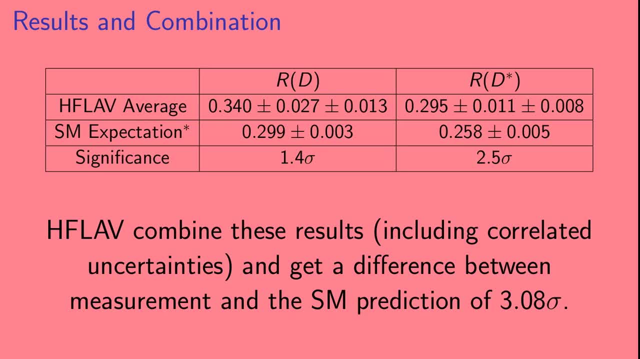 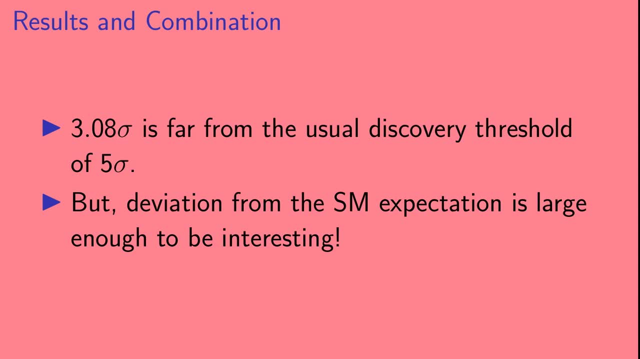 between measurement and the standard model prediction of the combined result of 3.08 sigma. Now, 3.08 sigma is far from the usual discovery threshold of 5 sigma, But the deviation from the standard model expectation is large enough to be interesting.